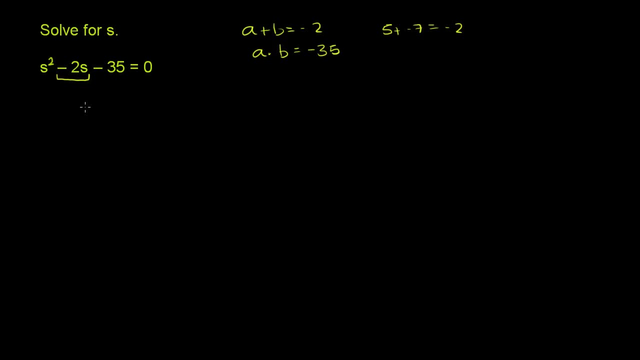 So to factor by grouping, you split this middle term into a. we can split this into a. let me write it this way: we have s squared and then this middle term: right here, I'll do it in pink: This middle term, right there, I can write it as plus 5s. 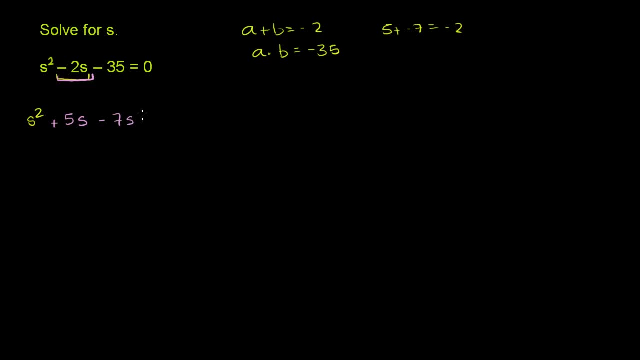 minus 7s, and then we have the minus 35. And of course all of that is equal to 0. Now we call it factoring by grouping, because we group it, So we can group these first two terms. And these first two terms, they have a common factor of s. 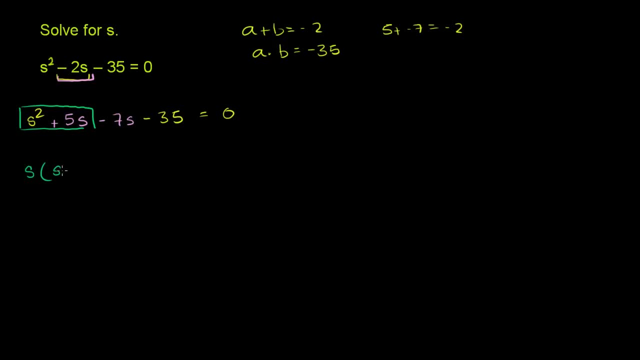 So let's factor that out. You have s times s plus 5.. That's the same thing. It's s squared plus 5s. Now, in these second two terms, right here you have a common factor of negative 7.. 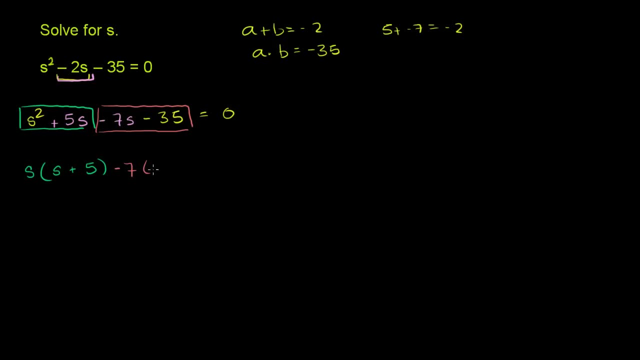 So let's factor that out. So you have negative 7 times s plus 5. And of course all of that is equal to 0. Now we have two terms here where both of them have s plus 5 as a factor. 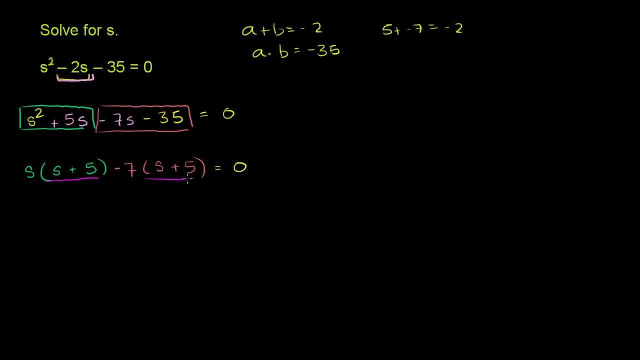 Both of them have this s plus 5 as a factor, So we can factor that out. So let's do that. So you have s plus 5 times this s times. this s right here. s plus 5 times s would give you this term. 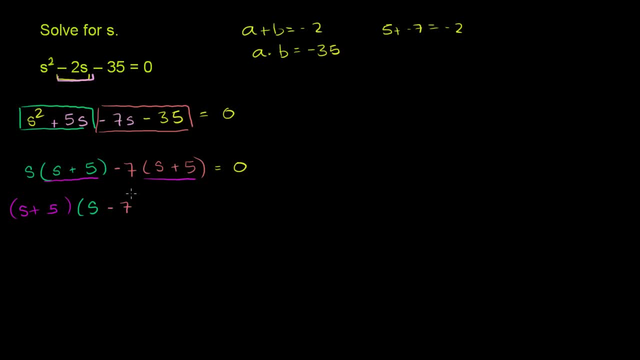 And then you have minus that 7, right there. I undistributed the s plus 5. And then this is going to be equal to 0.. Now that we've factored it, we just have to think a little bit about what happens when you take the product of two. 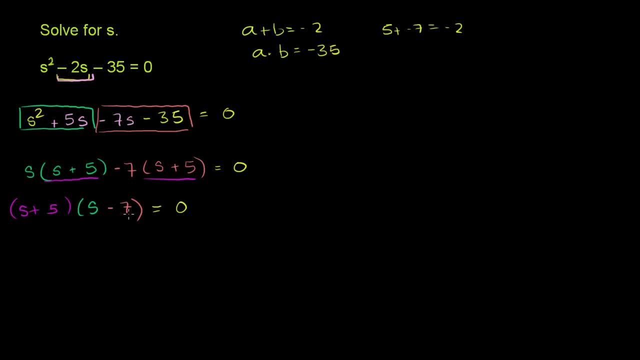 numbers. I mean s plus 5 is a number, s minus 7 is another number, And we're saying that the product of those two numbers is equal to 0.. If I were told you that I had two numbers, if I told you that I had the 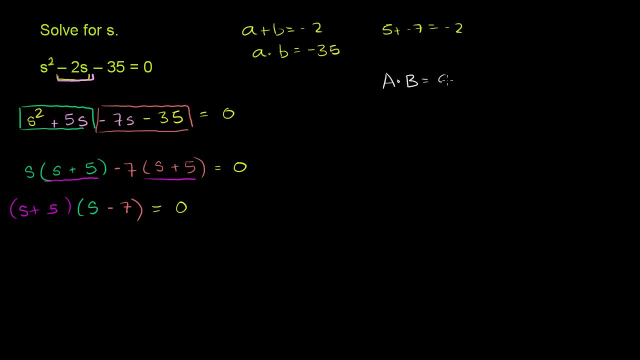 numbers a times b, and that they equal to 0, what do we know about either a or b, or both of them? Well, at least one of them has to be equal to 0, or both of them have to be equal to 0. 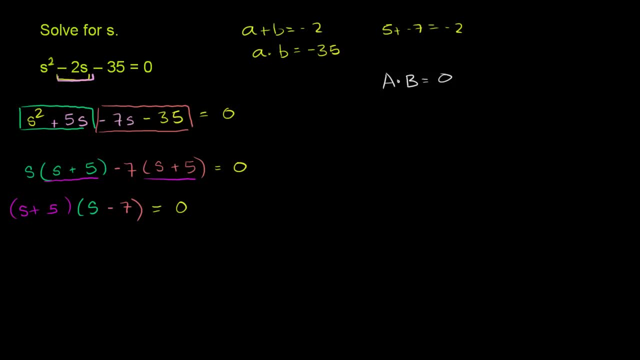 So the fact that this number times that number is equal to 0 tells us that either s plus 5 is equal to 0. Or, and maybe both of them, or s minus 7 is equal to 0, or I'll do that in just. 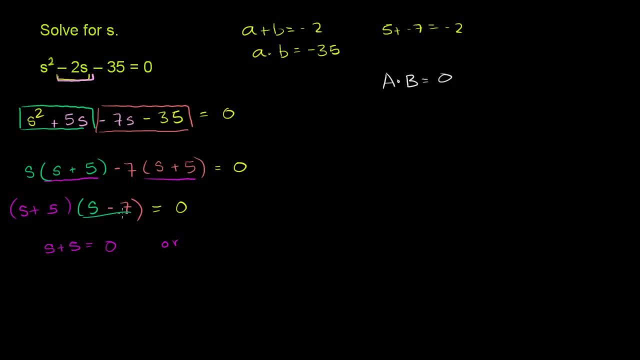 green, or s minus 7 is equal to 0.. And so you have these two equations and actually we could say and, or. It could be or and either way, and both of them could be equal to 0.. So let's see how we can solve for this. 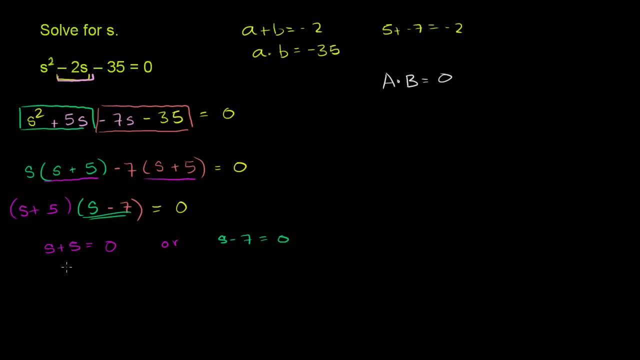 Well, we can just subtract 5 from both sides of this equation right here. So let's do that, And so you get on the left-hand side. you have s is equal to negative 5.. That is one solution to the equation. 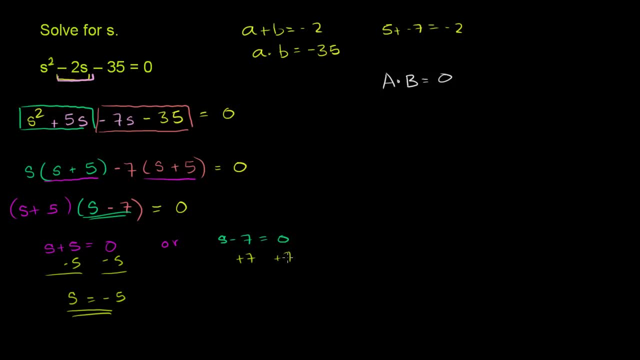 Or you have. let's see, you can add 7 to both sides of that equation And you get s is equal to 7.. So if s is equal to negative 5, or s is equal to 7,, then we have satisfied. 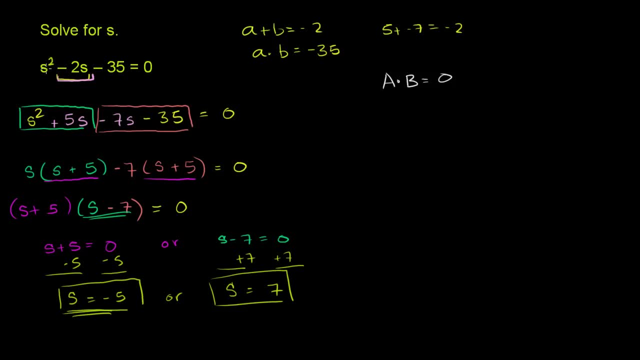 this equation. We can even verify it. If you make s equal to negative 5,, you have positive 25.. Plus 10,, which is 35, minus 35,, that does equal 0.. If you have 7,, 49 minus 14, minus 35 does equal 0. 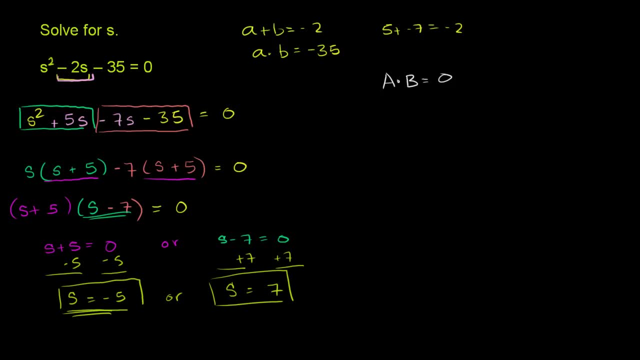 So we've solved for s. Now I mentioned there's an easier way to do it, And when you have something like this, where you have 1 as the leading coefficient, you just you don't have to do this two-step factoring. 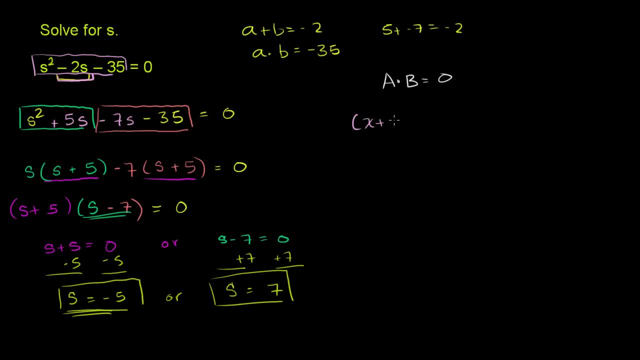 Let me just show you an example. If I just have x plus a times 0.. X plus b, what is that? equal to X times x is x squared. X times b is bx. A times x is plus ax. A times b is ab. 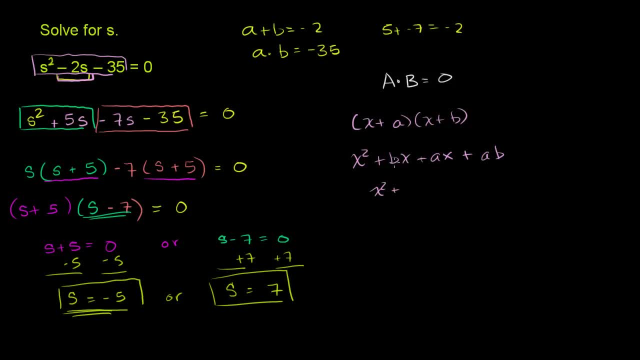 Plus ab, So you get x squared plus. these two can be added: plus a, plus bx, plus ab, And that's the pattern that we have right. here We have 1 as a leading coefficient here. We have 1 as a leading coefficient here. 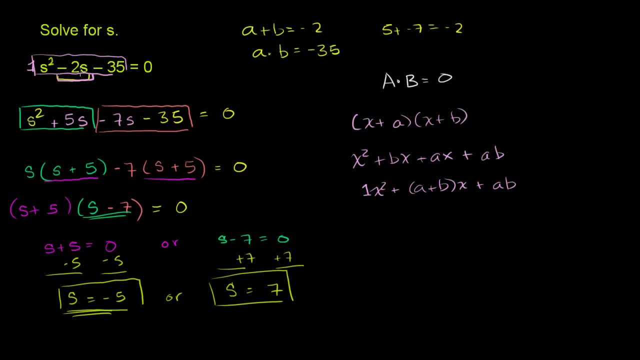 So once we have our two numbers That add up to negative 2, so once we have our two numbers that add up to negative 2, that's our a plus b And we have our product that gets to negative 35. Then we can straight just factor it into the product of those two things.